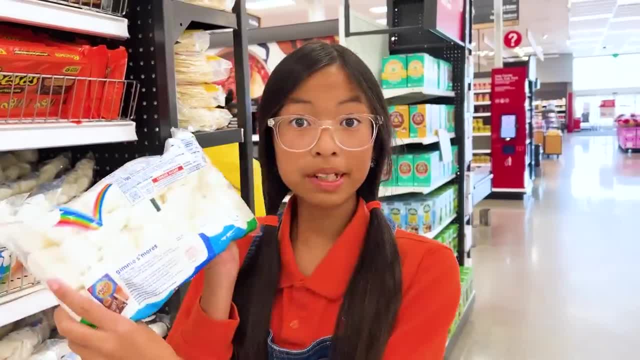 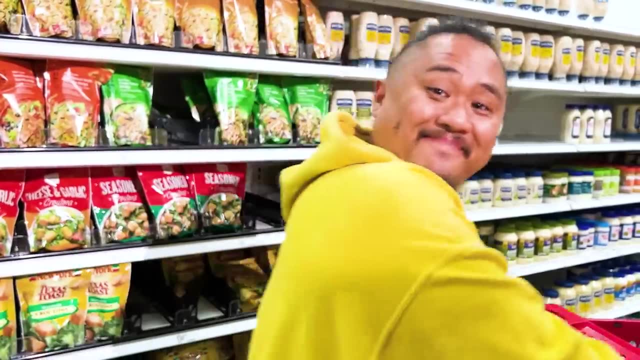 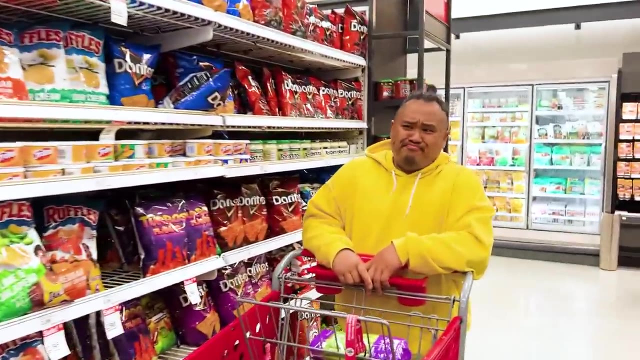 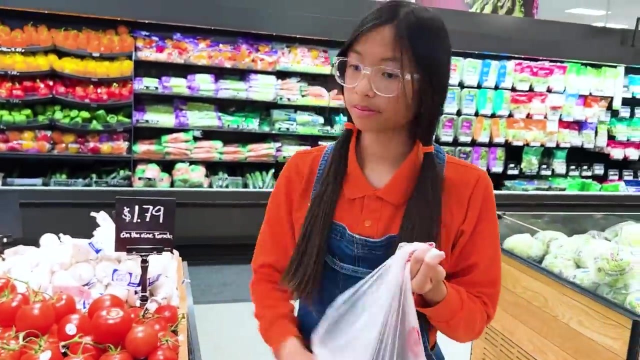 Oh, how about soda? How about water? Marshmallows? Put it back. Get the bread, Wendy. Okay, Oh, chips. There's better things than chips, Wendy. Tomatoes are better. So I told you There's water there, Wendy. 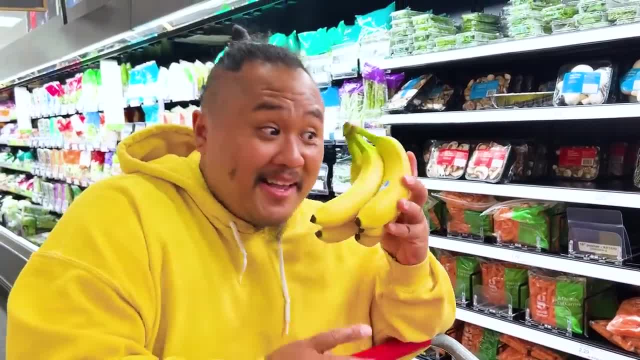 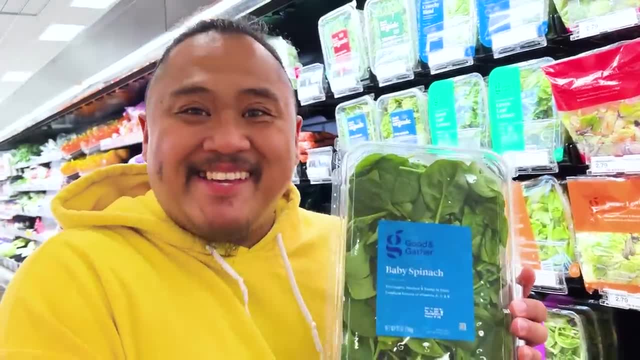 Oh, Bananas have a lot of potassium. Oh, healthy, Awesome Spinach has vitamins A, C and K. Wendy, do you know? celery is good for your brain. I want something good, But, Wendy, these are grapes. 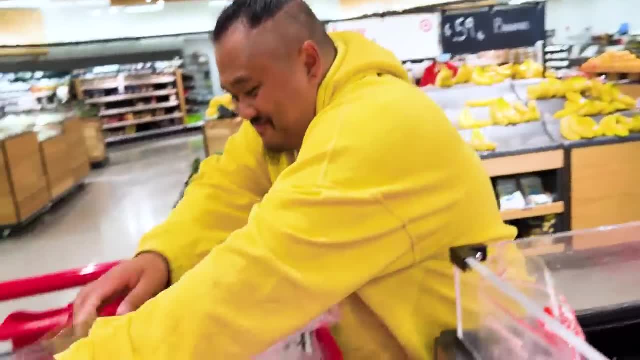 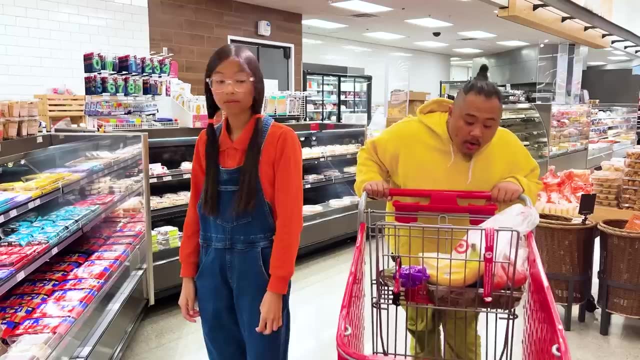 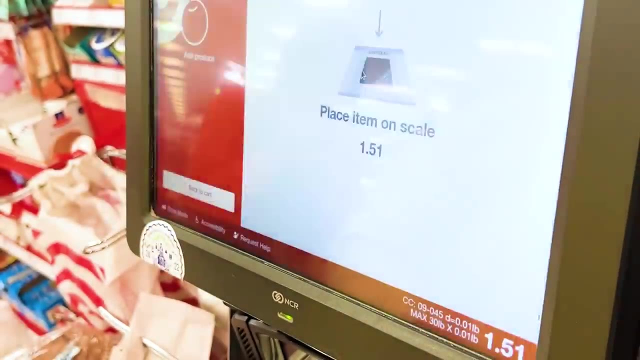 Grapes. They're seedless. Oh, how about cake? You know what's better? Apples, Cool. Oh, looks like we got everything we need: Snacks, Cupcakes, Yes, Ah. Oh, your bath, We got the groceries. 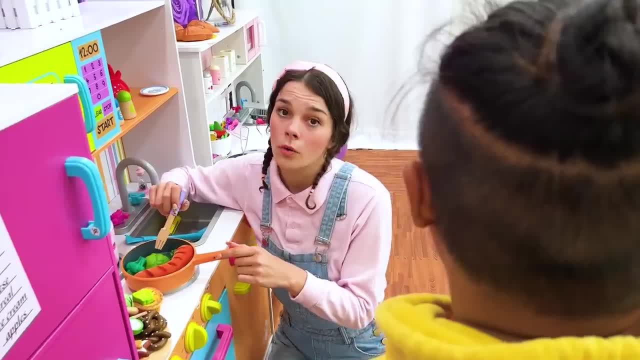 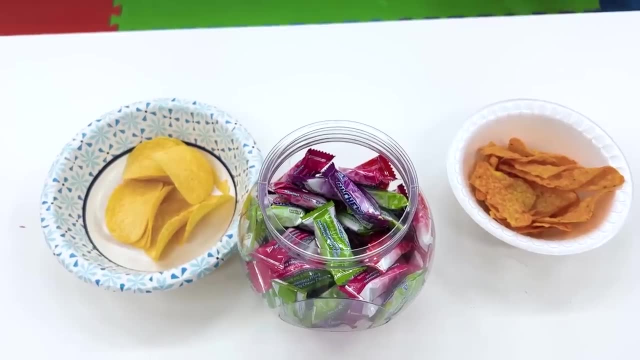 Why does Wendy seem so disappointed? All she wanted was junk food. Oh, I see I'll be in another room. Ah. Ah, Wondy, are you okay? I just got back from the grocery store And Uncle Sam. 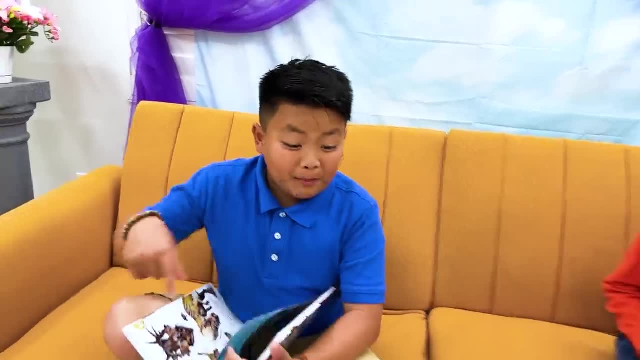 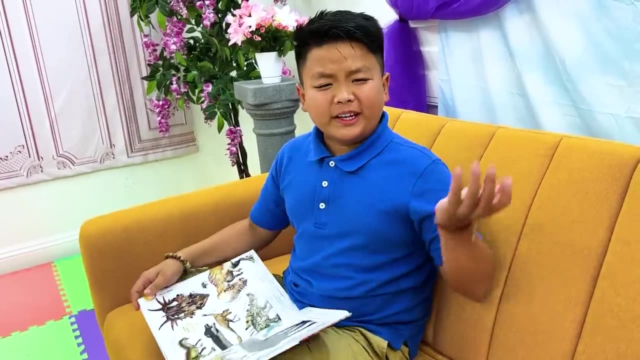 Wait, Wondy. no, Huh, No tofu. Sorry, Uncle, I meant to clean that up. Wondy, what are you eating? I hope those were carrots. I only had one chip. Here's some fruits. 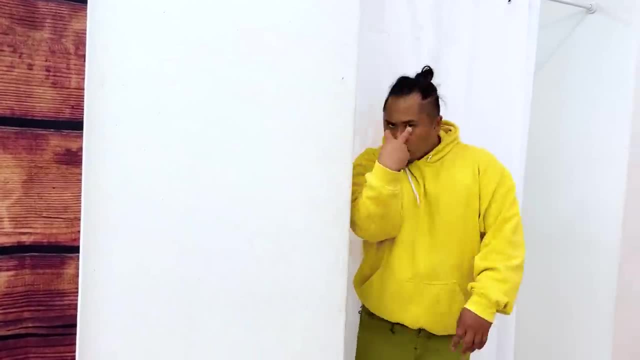 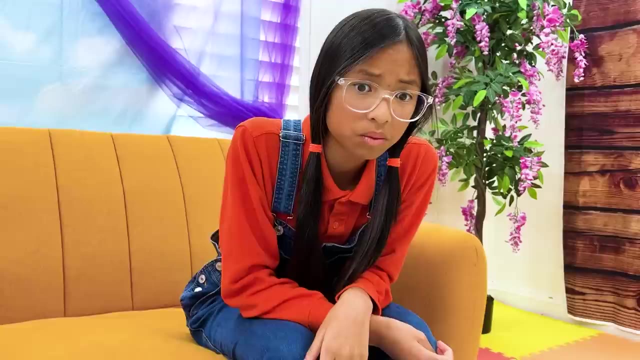 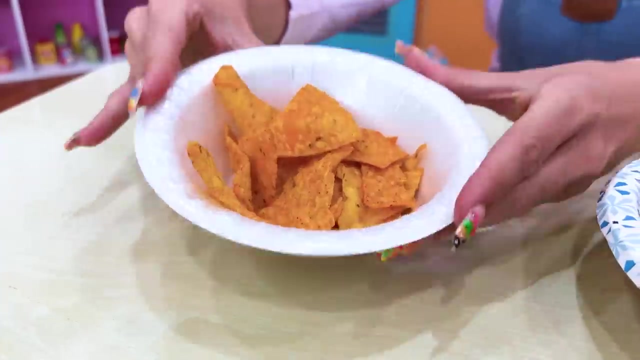 It's good for you. Ooh, Have some fruit, It's good for you. No, thanks, Whoa, I don't crave for junk food anymore because I eat fruits. Wondy, Alex, We need to slow down on buying chips. 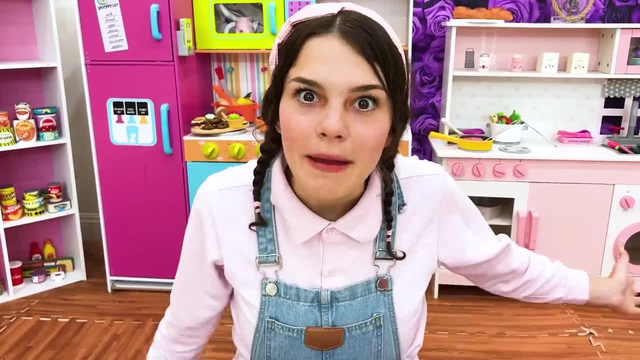 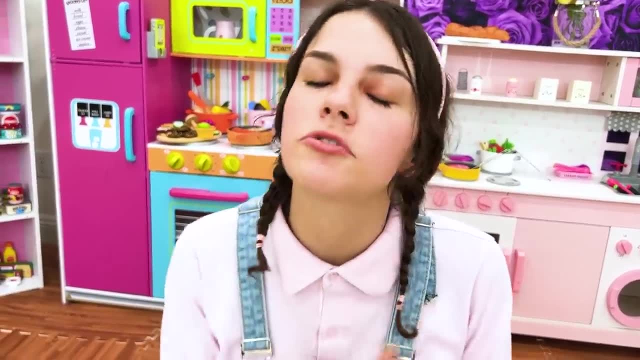 Hey kids, I have some grapes. We should make more healthy snacks. Yeah right, Wondy, This isn't grape. Huh, These are cheesy. A chip must have fell in there. I'm so sorry, Wondy. 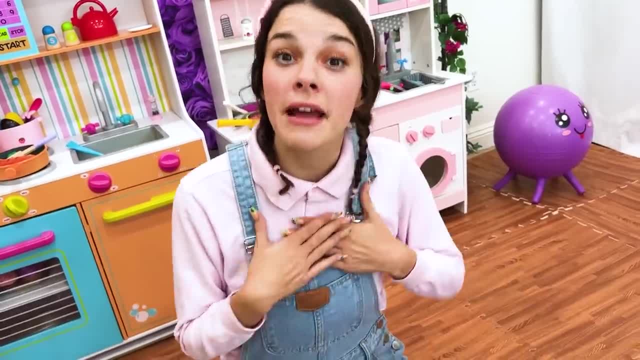 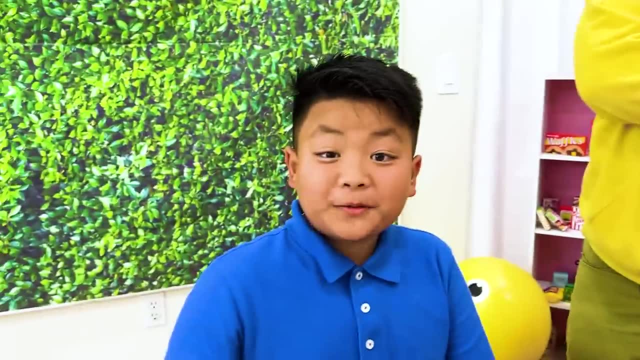 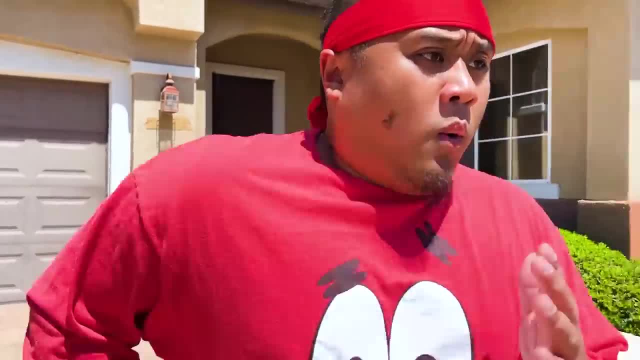 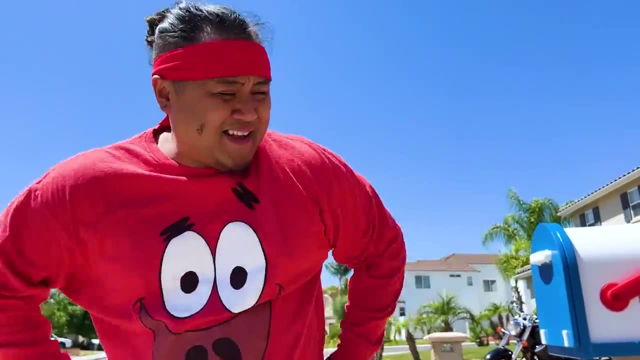 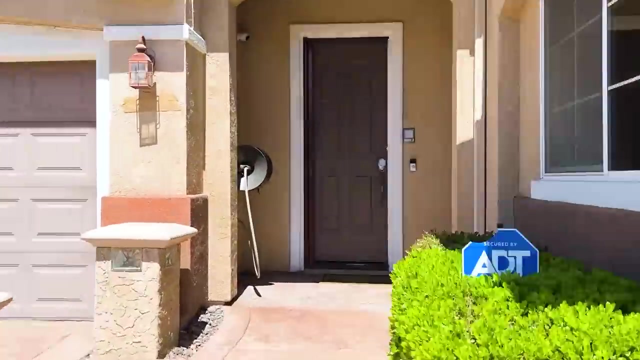 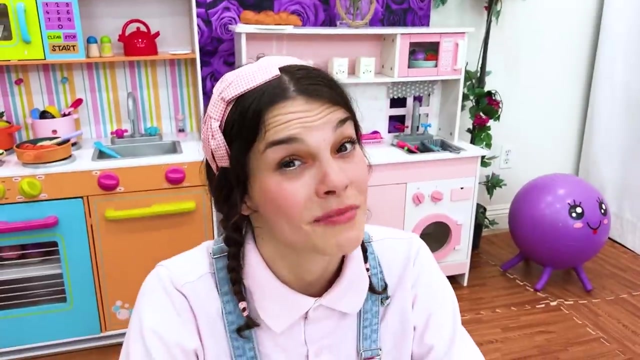 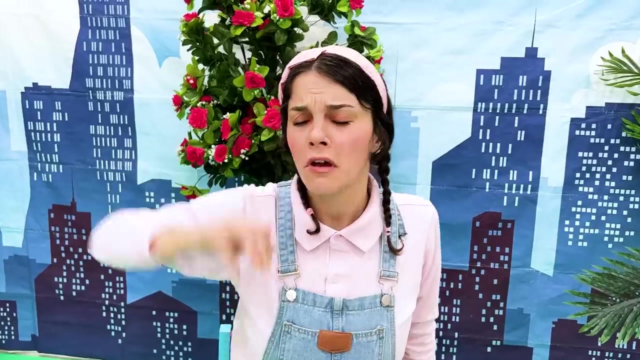 Mmm, Mmm, Mmm, Mmm. New record. Well, time to get back. That's a long way. Let's go Really. Yep. Oh, Same thing happened to me. Awesome Yum, I'm so full. 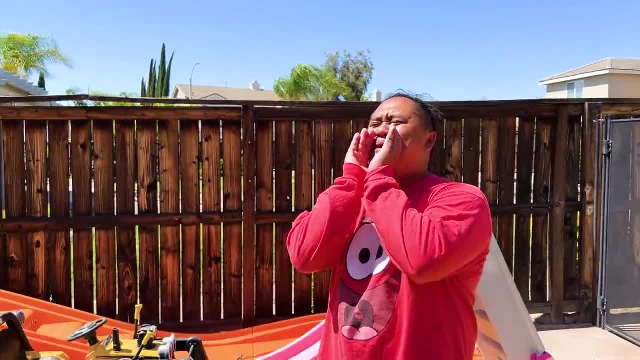 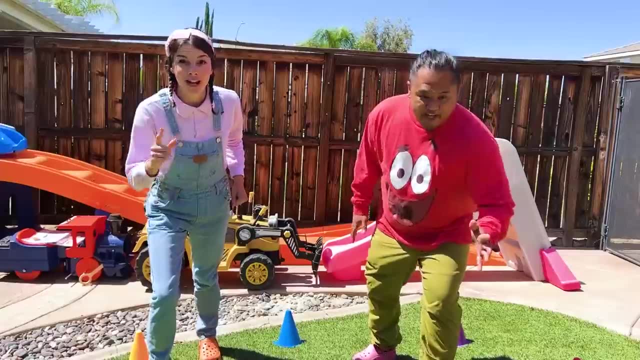 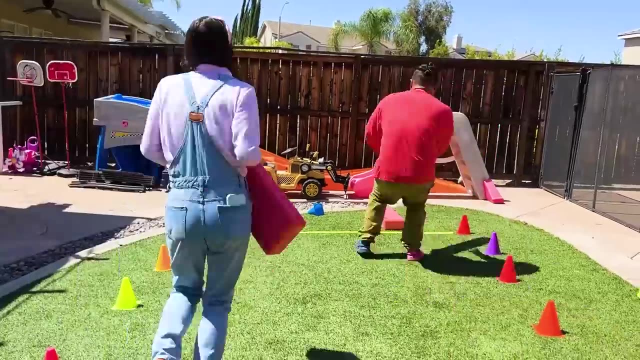 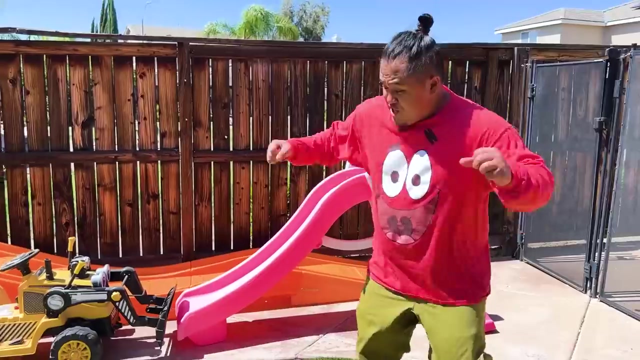 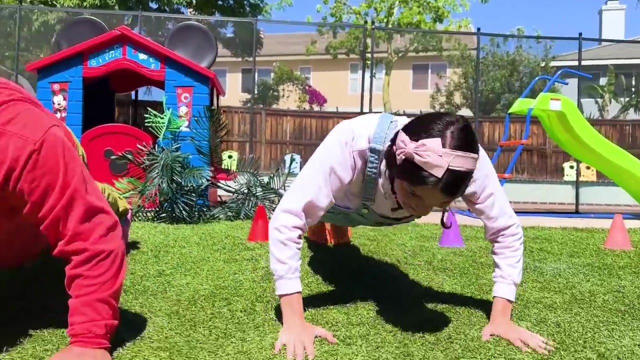 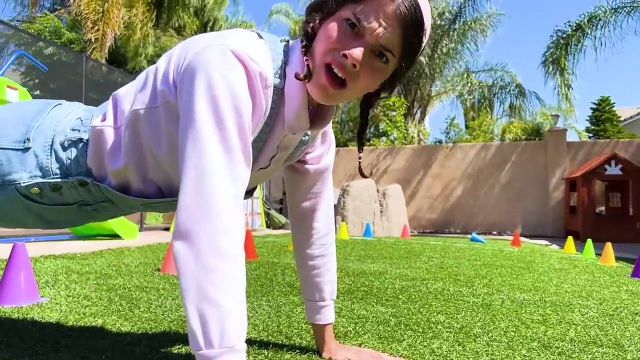 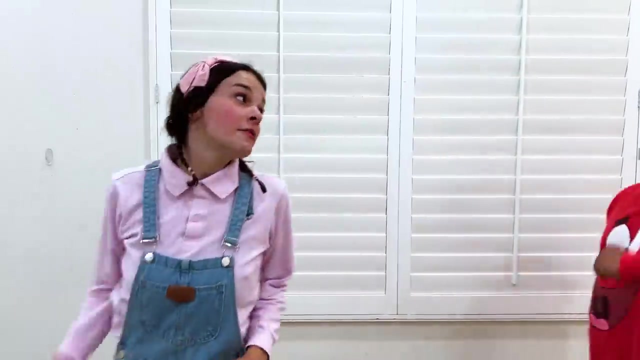 Auntie May, I'm here, Ready to race. Okay, Ready set, go. Yeah, Push-up competition, ready, Go? How are you doing that? Looks like I'm winning, You win. That was a fun competition. How did you get so fast? Well, here's some fruits. 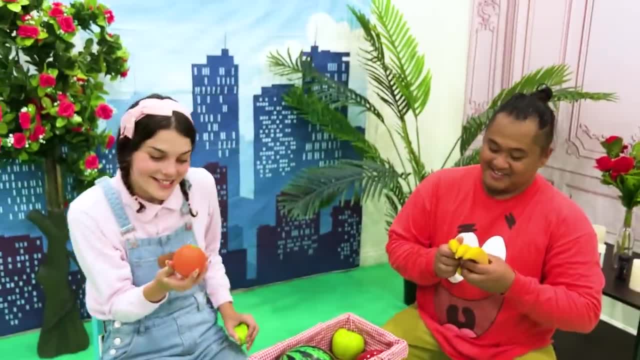 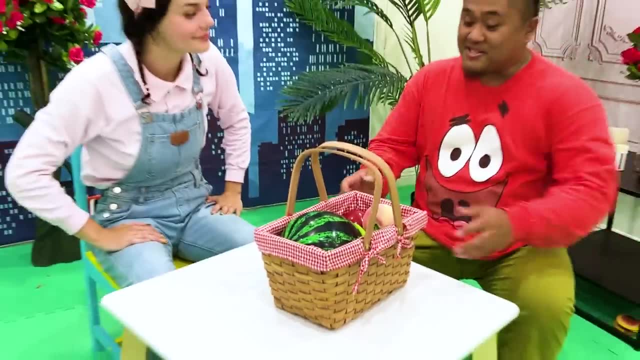 It'll help you with your stamina. I'm gonna have some bananas, An apple. Apples- it gives you a lot of energy. Oranges: they have a lot of vitamin C. That was so good. You wanna play another game? Yeah, let's go on a bike race. 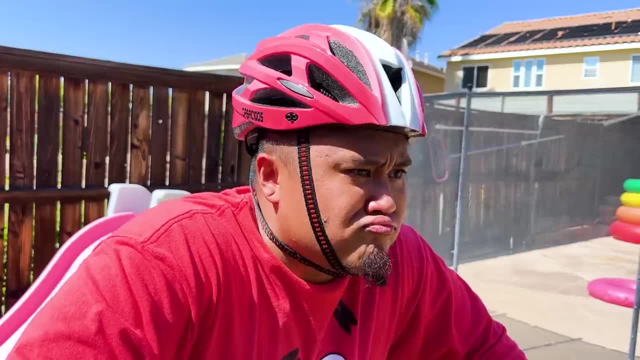 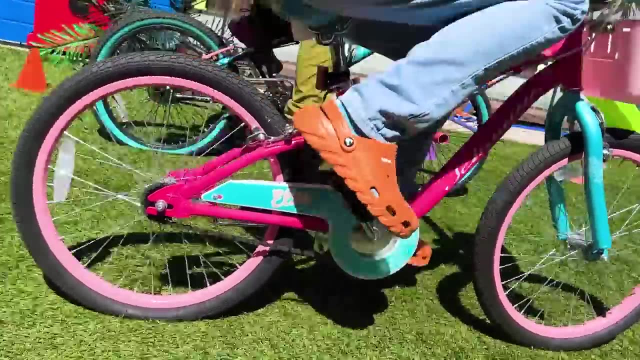 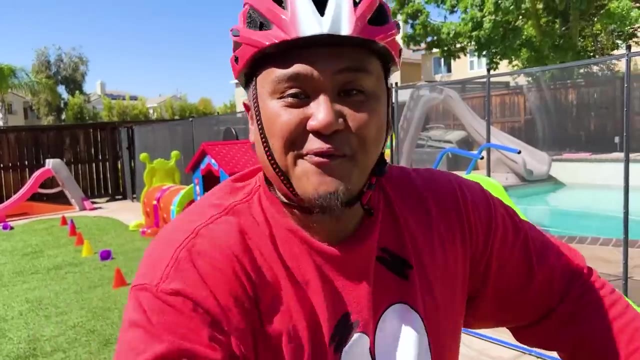 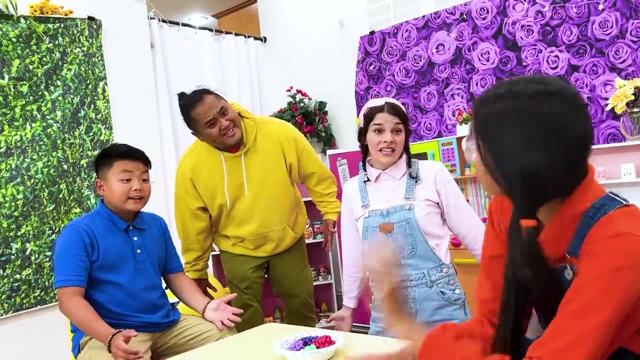 I'm gonna win this time. Are you sure I'm gonna win? Yay, Good job. I told you fruits and vegetables will help. You're right, thank you. And it's All because of junk food, Wendy. Oh, sorry, Maybe you should take a nap. Good idea, sorry again. 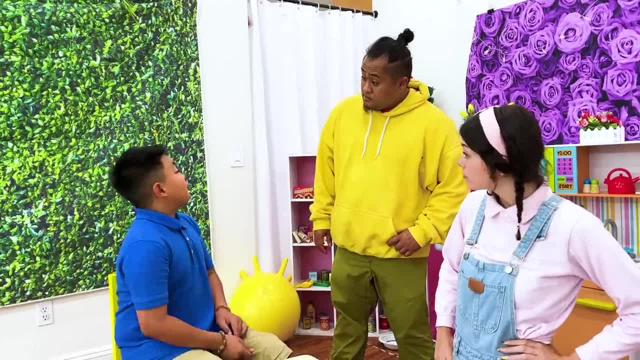 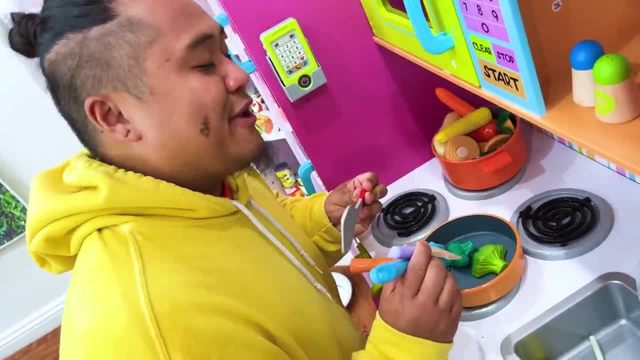 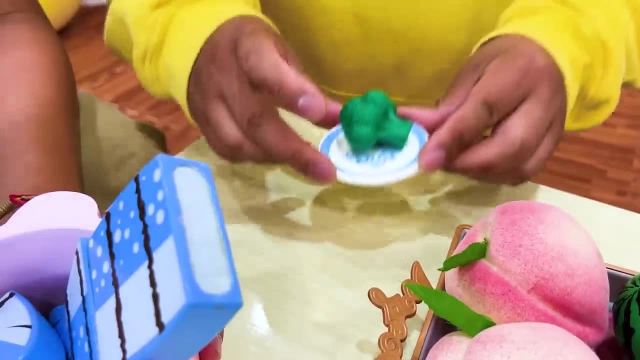 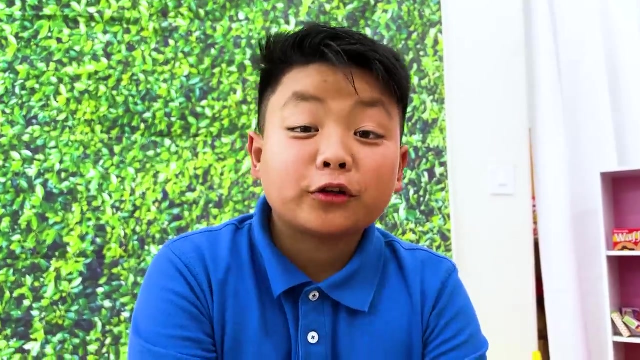 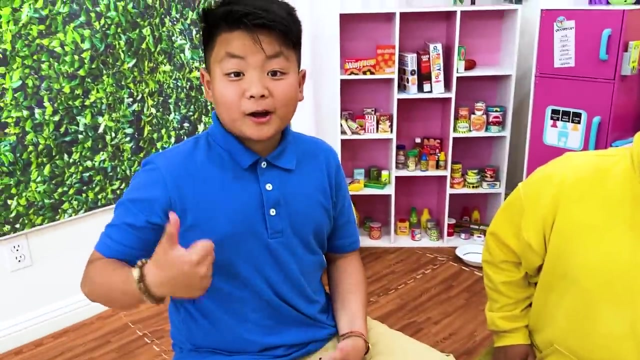 We should prepare alternatives for junk food. Great idea, Awesome, Hi. Wow, look at all this food. Yeah, It's a healthy alternative. Wow, Wow, it's so colorful like candy, But it's healthier And better. You did all this for me, Thank you, You're welcome. Bye.